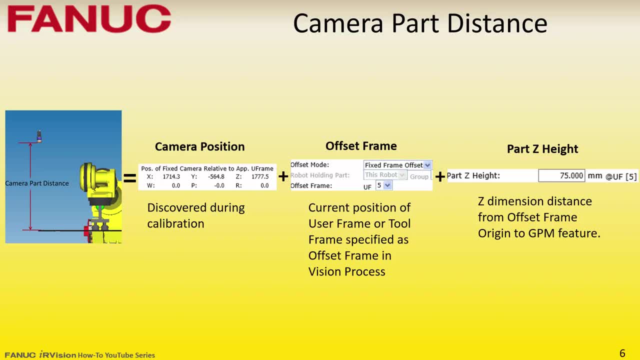 during calibration, the current position of the offset frame and the part z-height, which is entered by the user. Using these three values, IR vision can accurately calculate the camera-to-part distance. By calculating the camera-to-part distance in this way, the user is not required to directly. 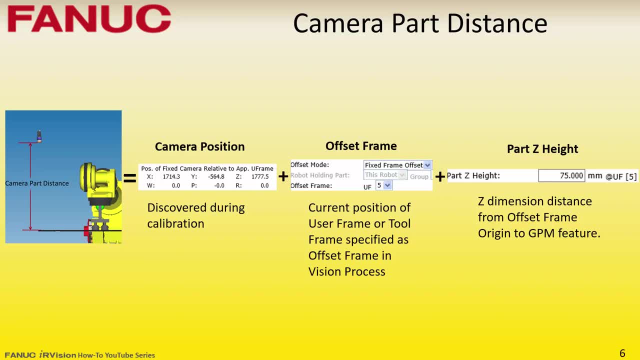 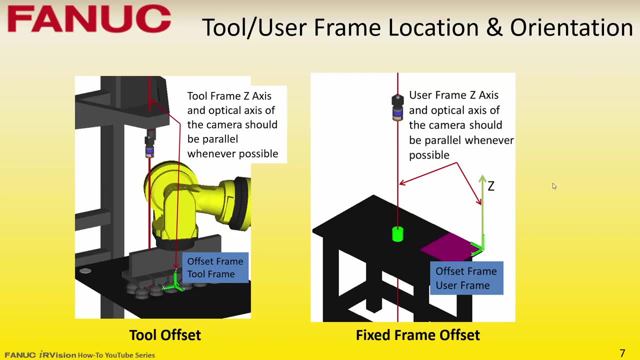 measure the camera-to-part distance, which would be very difficult to do accurately. When possible, the offset frame, z-axis and the optical axis of the camera should be parallel. With perspective calibration, IR vision can accurately calculate the camera-to-part distance. In perspective calibration, the camera can be at an angle to the offset frame and accurate. 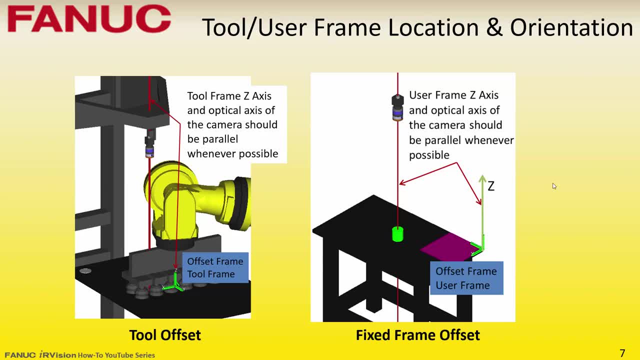 information is still calculated. The z-axis of the offset frame can point away from or towards the camera, The tool frame or user frame. origin location can be anywhere but the distance from the origin of the offset frame to the part feature being located by the vision process needs. 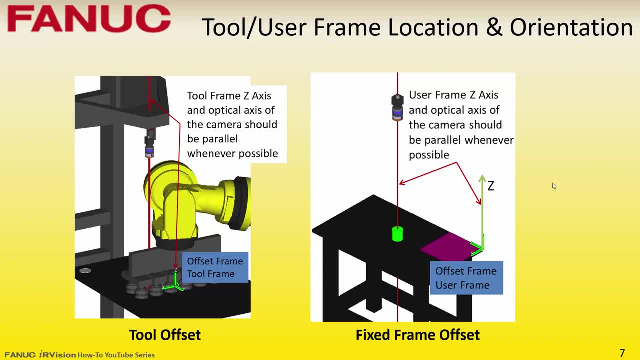 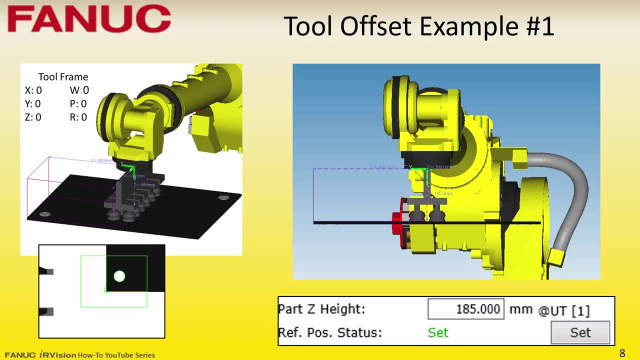 to be known in the z-dimension only and entered as the part z-height. In this first tool offset example, using a zero tool frame and a part that is positioned 185mm away from the faceplate, the part z-height would be positive 185mm. 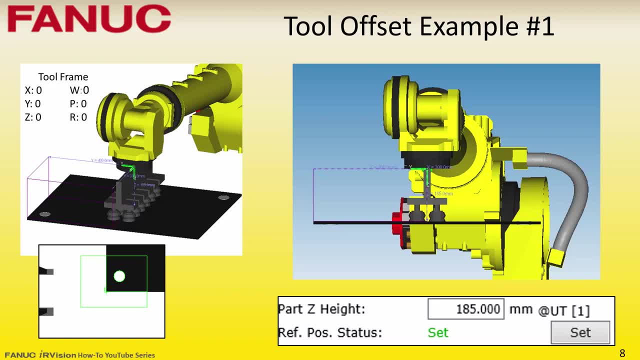 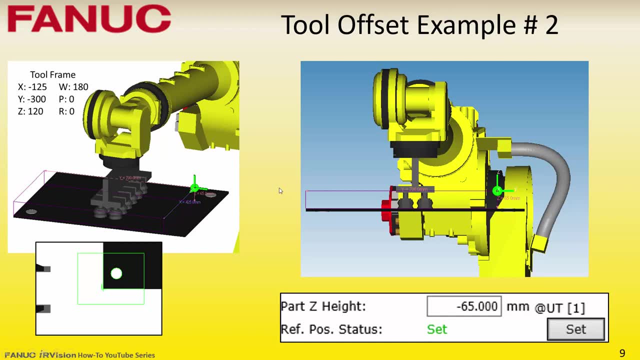 The part z-height is positive because the z-axis points out of the faceplate. In this second tool offset example, the tool frame origin is moved to some random location and the orientation of the tool frame is changed such that the z-axis points up. 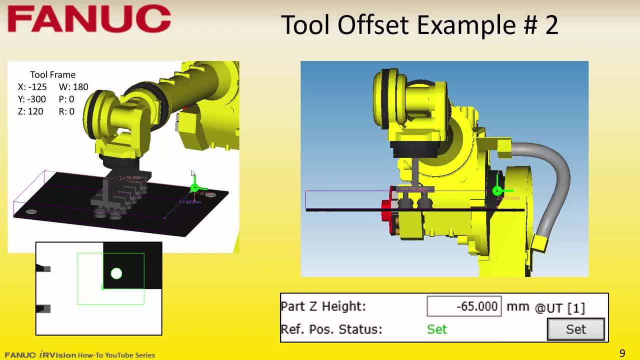 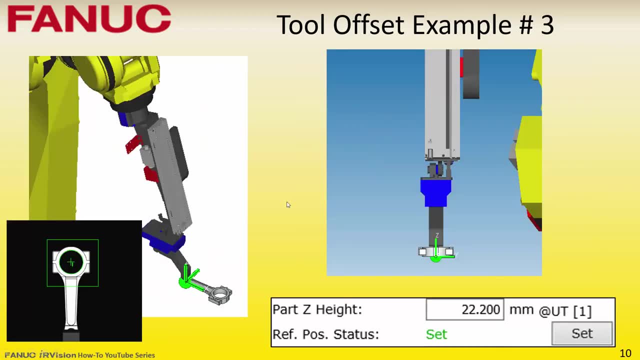 The part z-height for this case is negative- 65mm. The z-axis points out of the faceplate. The part z-height is negative because the z-axis points up and the feature is located below the TCP. For the third tool offset example, the part is held at a 15 degree angle from the robot. 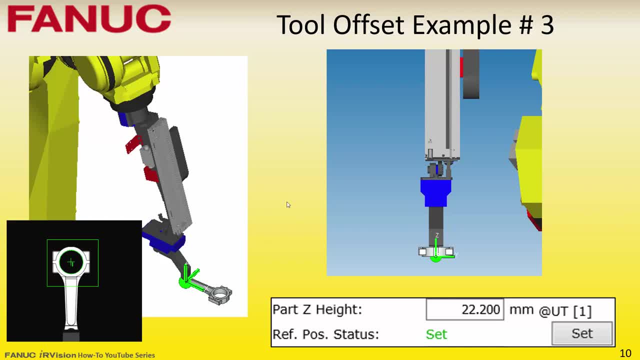 faceplate and the orientation of the tool frame is such that its z-axis is in line with the optical axis of the camera. The correct part z-height for this example is positive 22.2mm, because the tool frame origin is located 22.2mm below the feature being located and the z-axis points up. 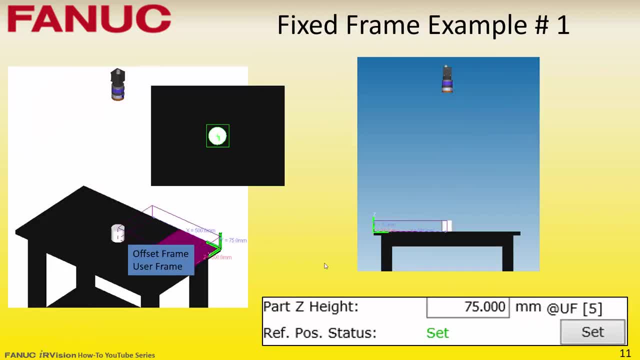 To the camera. In this first example of a fixed frame offset, the offset frame user frame has been taught to the top corner of the table with the z axis pointing up towards the camera. The part z-height for this vision process will be 75mm, which is the height of a part.